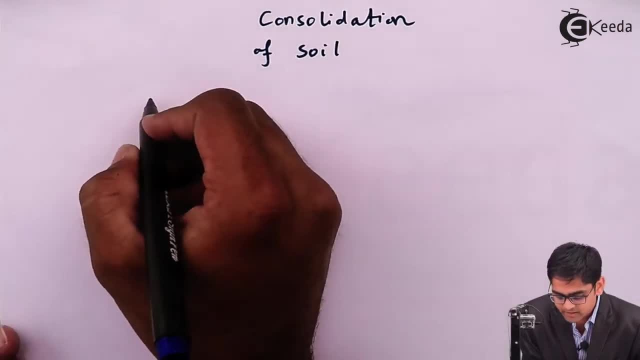 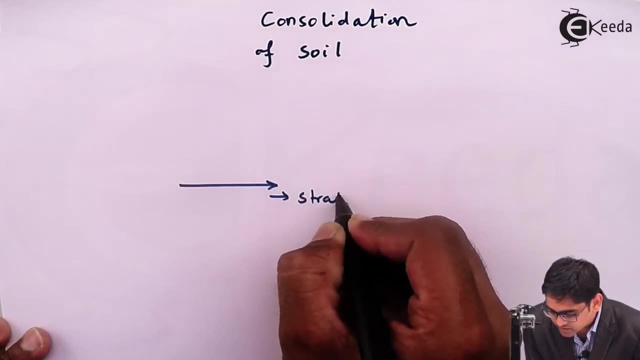 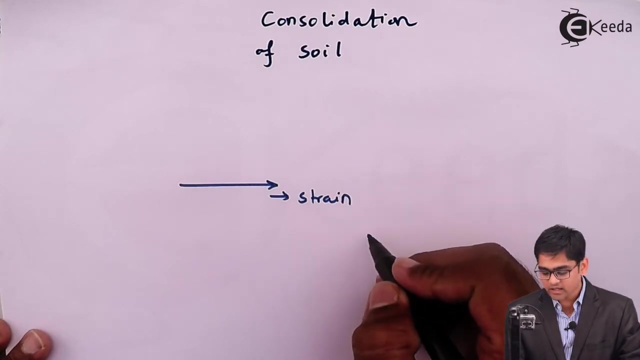 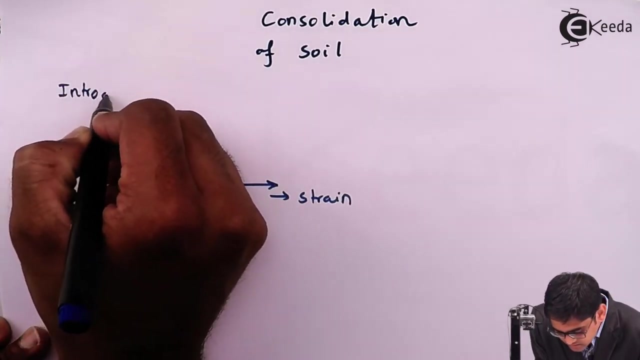 for all convention analysis, we plot the strains on the x-axis. These strains may be the axial strains, may be the shear strains, or may be the distortion angle which is caused because of the shear forces. So, and on the y-axis, we plot the shear forces, So the shear. 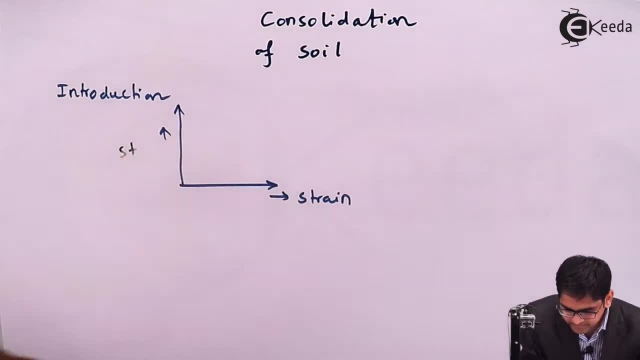 forces that will be nematodisc confusing and the strain will be gone. this is what we are talking about. So if I take an example of a phase of scare strain that is SAL SW, let us take this truck. we will be plotting the values of stress. 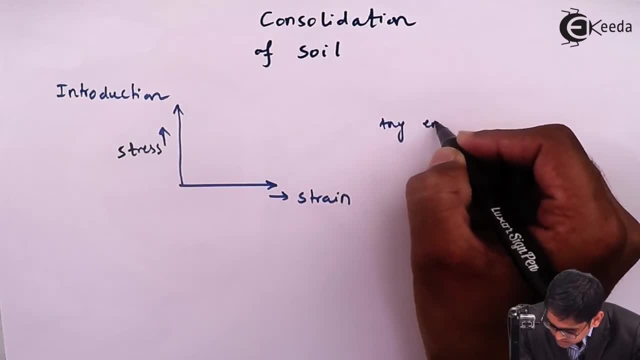 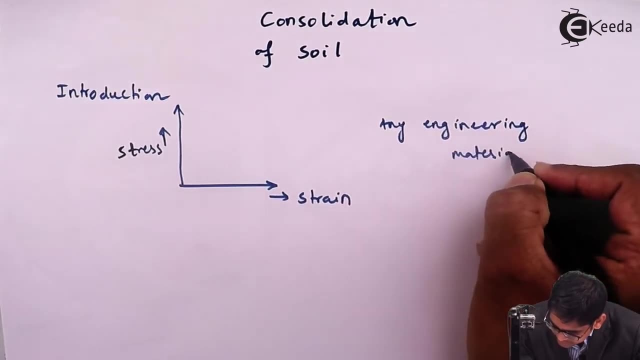 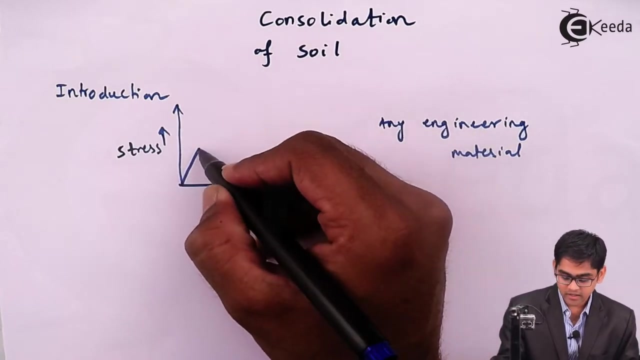 And if you take an engineering material- may be a concrete or a steel- you will get the response of the electric curtain in curve. initially you will get it has a straight line and there you have several chains, current lines and differentsto, a under- longevity duration. 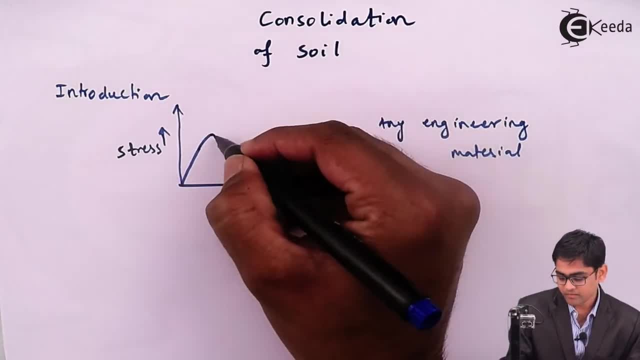 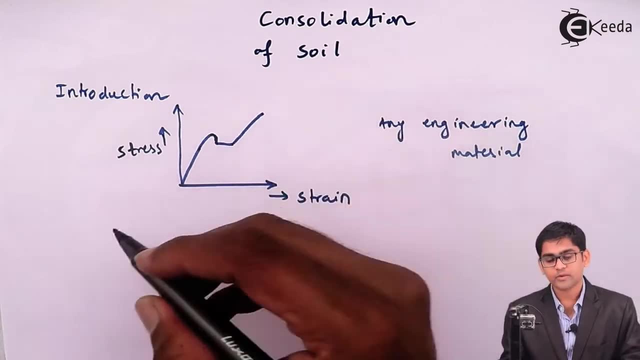 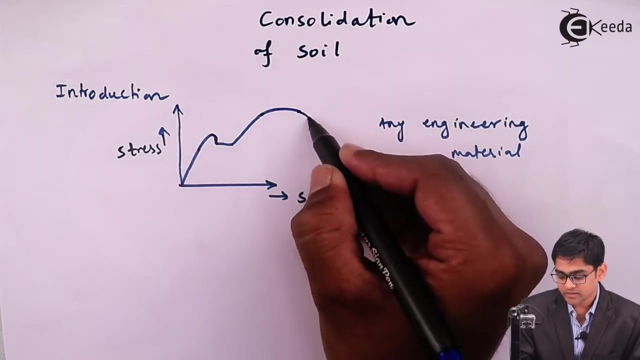 it will reach the value of upper yielding point and then lower yielding point, then a softer response or then, probably because of the reorientation, you will get the increased strength of the material and after reaching ultimate value, it ultimately breaks over this point. So B is the breaking point. 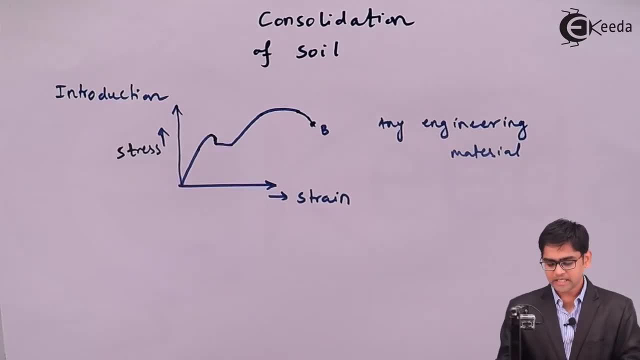 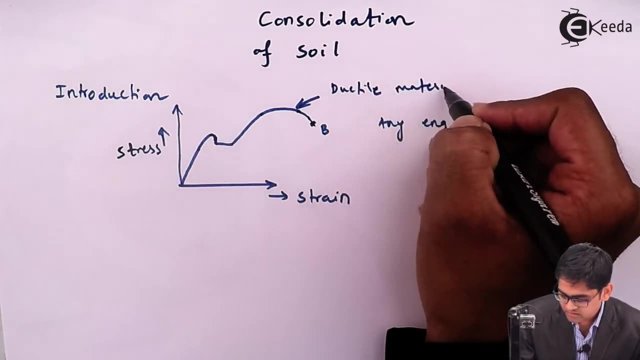 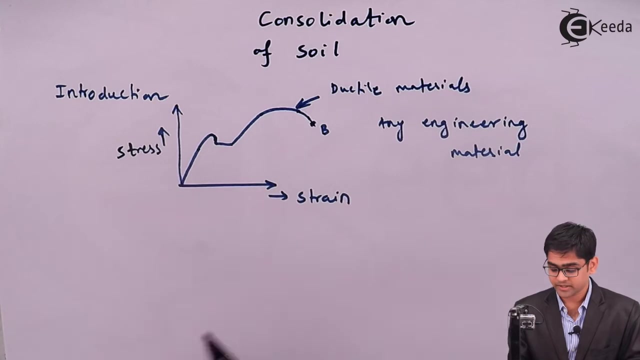 So we saw this kind of particular curve for ductile mild steel. this is for ductile materials which go on continuously straining while developing the internal resistance against deformation. So this ductile material example is mild steel and if you compare it with the concrete which 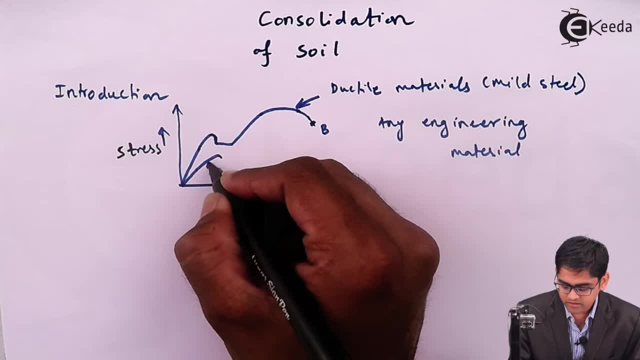 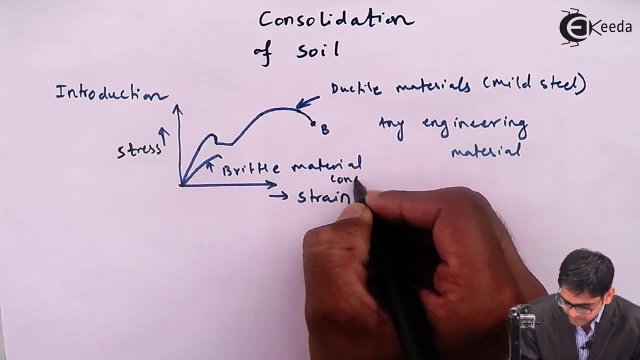 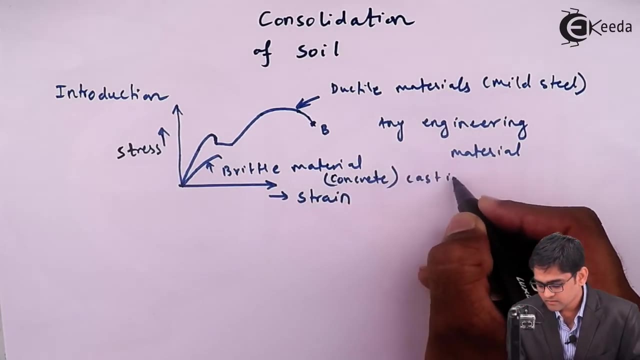 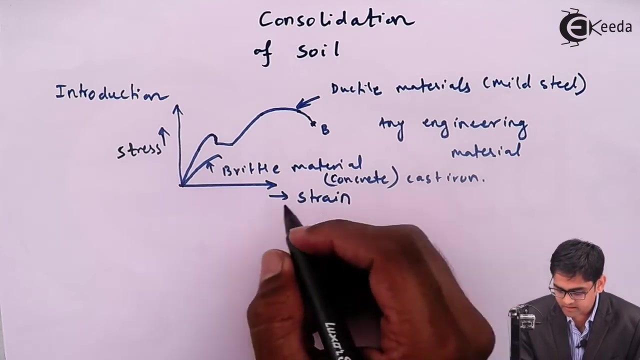 is kind of brittle response. so this is for the concrete. for brittle material May be the concrete or may be the cast iron, there are various engineering materials and you will. you have seen such kinds of the response of the material under the application of load. 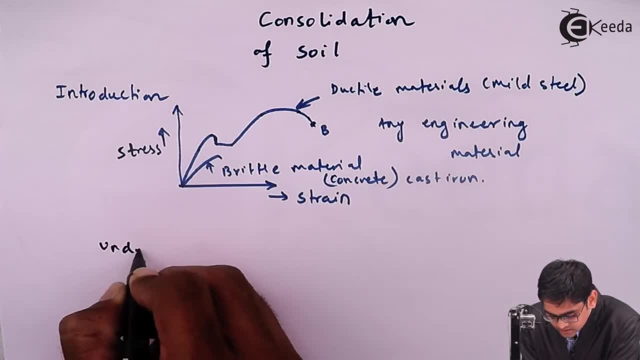 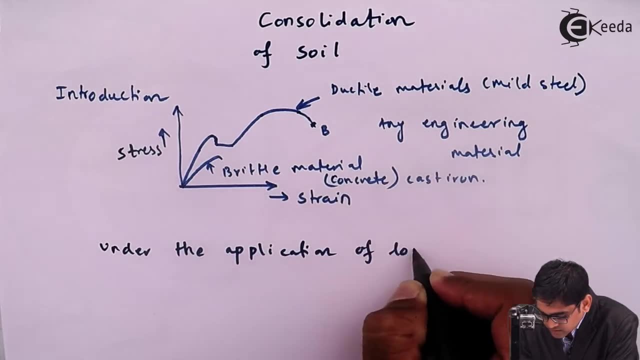 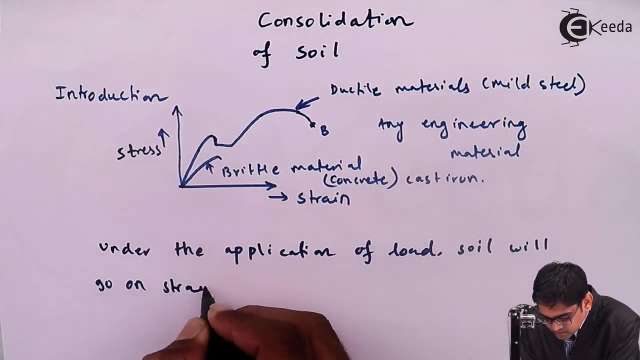 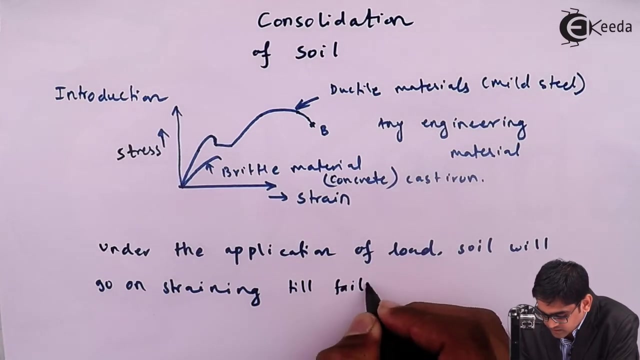 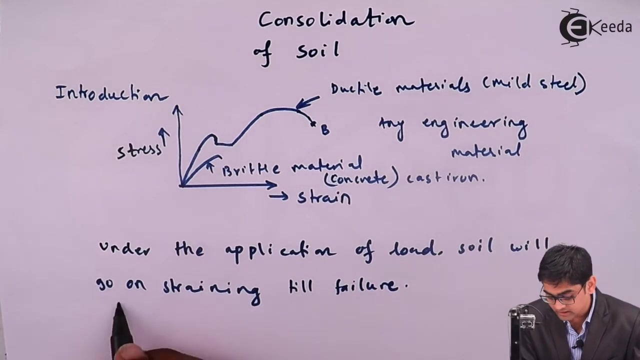 So it is. so I will write over here- that under the application of load, Soil will go on straining till failure, till failure. But what happens in most of the cases as far as the soil is concerned? so if you draw, particularly the stress, strain curve. 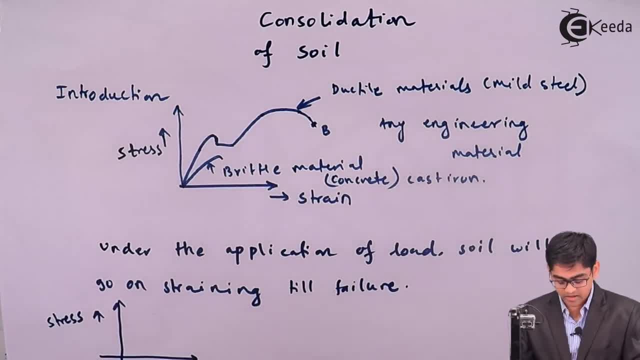 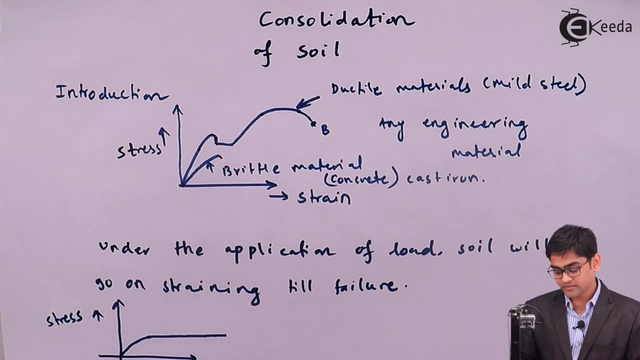 For, For, For Obviously, I will here discussing only the axial stresses and axial strains. So the soil will go on straining and straining, straining, but it will not fail. So here for such kinds of material, which is for loose sand or for I call it as a normally 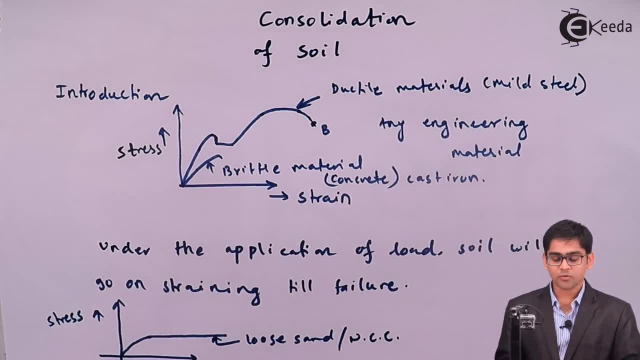 consolidated clay we will see such kinds of the stress strain response in the shear strength of the soil. So this is for the soil chapter and for the dense it's like this one. this is for a dense sand or over consolidated clay. So this OCC means over consolidated clay. 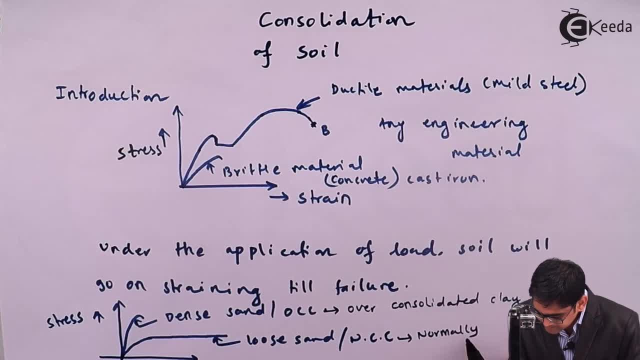 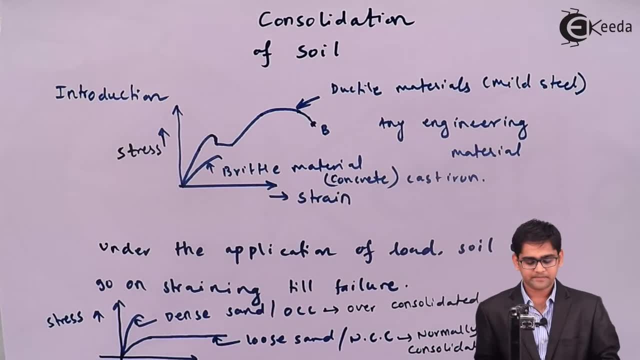 And NCC means normally consolidated clay, Okay, Okay, Okay. So this is for滕. So we will use the same Shrink원이 method, Shrink wifi method for the unstable爸爸 vsды method. It's a programmed formula. 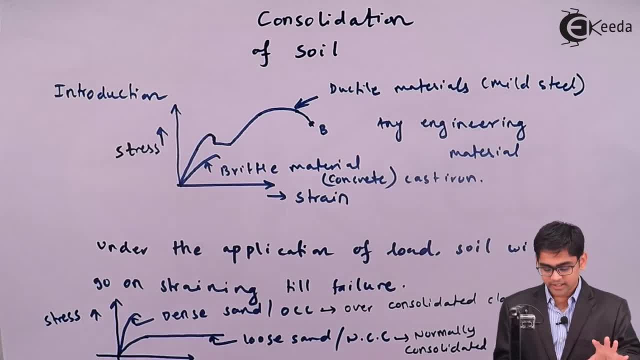 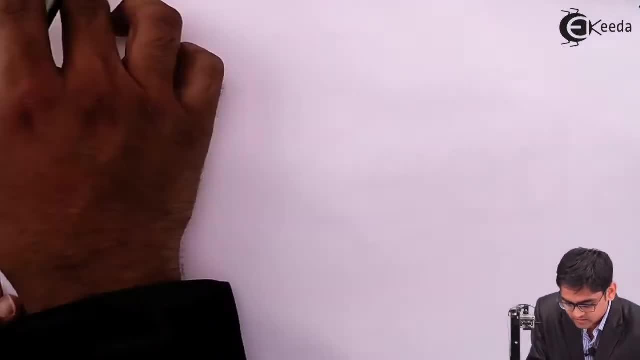 They, they do not need water and soil. They know that they want to create a simple surface. So these 3 don't want to create MUSIC. These backup now is that? properties of the soil: first, it is very, very important, which is nothing but the soil type. 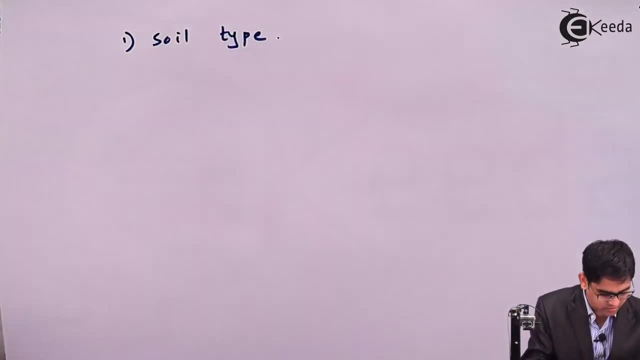 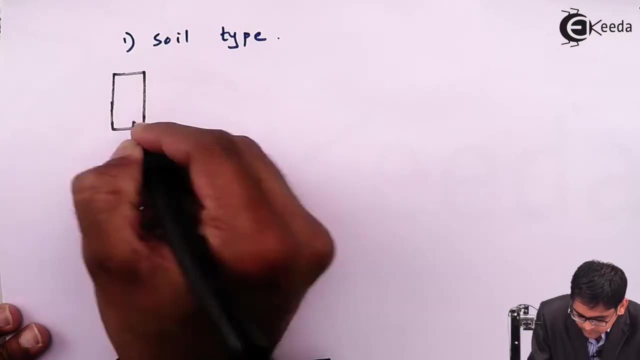 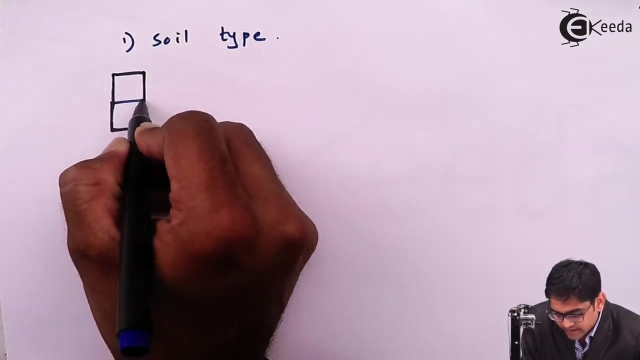 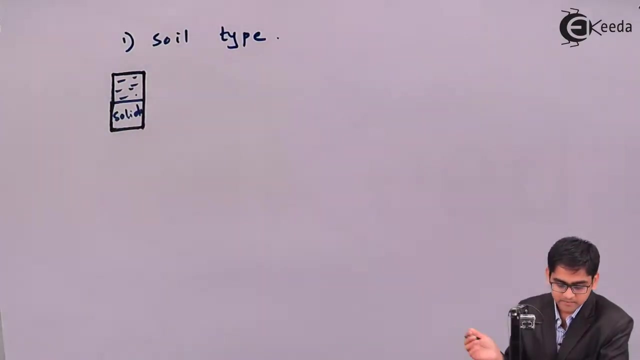 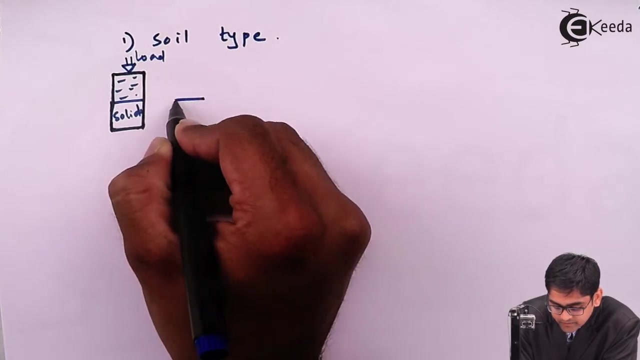 so, as we have seen that, particularly in case of a clay deposit, we have got the solids and clay is almost in all general cases it is fully saturated, and once you up the load it to a clay soil then, since the solid part, is the incompressible. 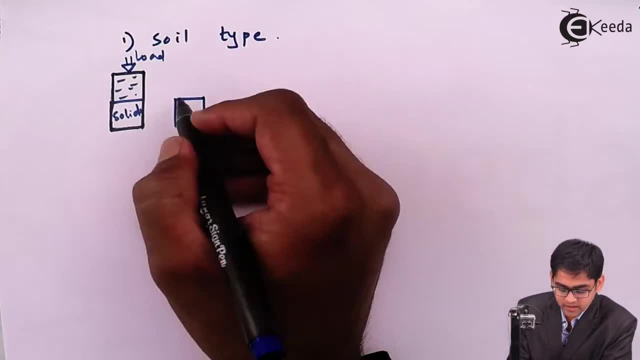 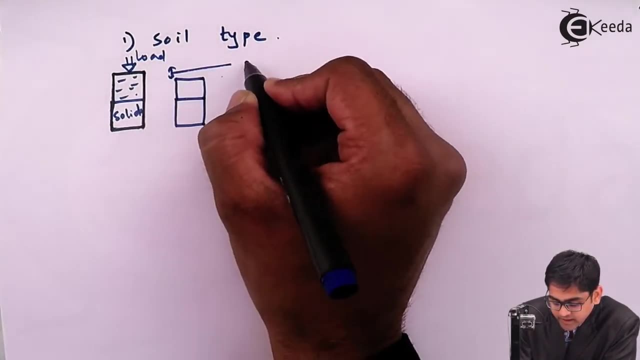 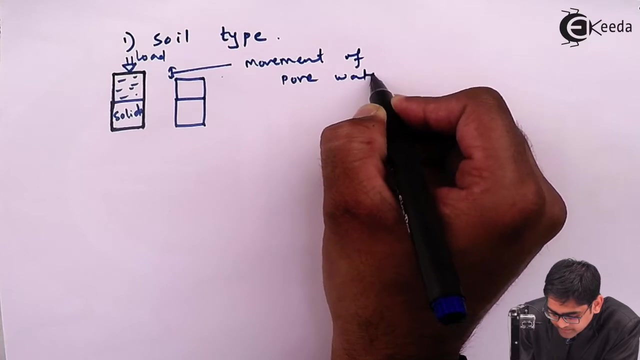 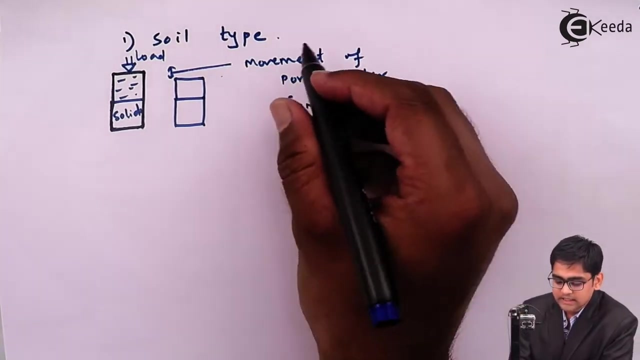 the volume change will not occur into the solid. the volume change will occur only in case of the voids. so it will happen because of the movement of water- or I call it a moment of poor water- from its structure and this is happened because of the load. so very, very important this moment of the 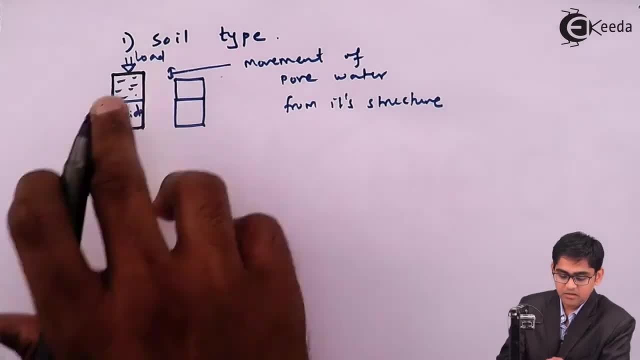 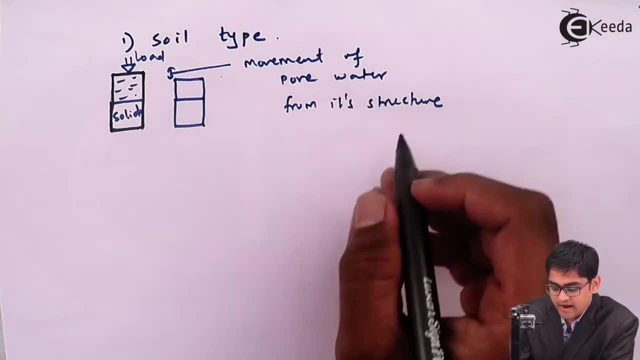 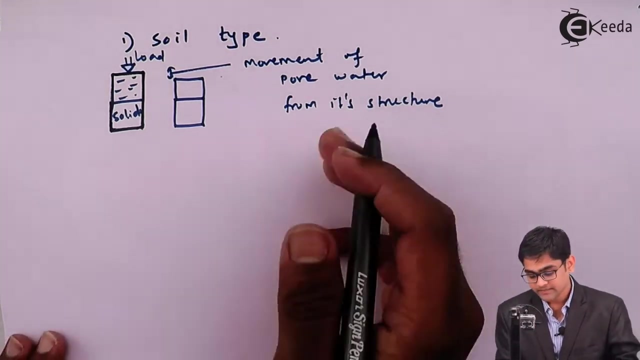 poor water has happened because of the load. how it has happened, see, in order to have, in order to have the movement of the poor water, or for a seepage, we must, we have studied that it is must for us to generate a difference in the total head then, and then only the flow. 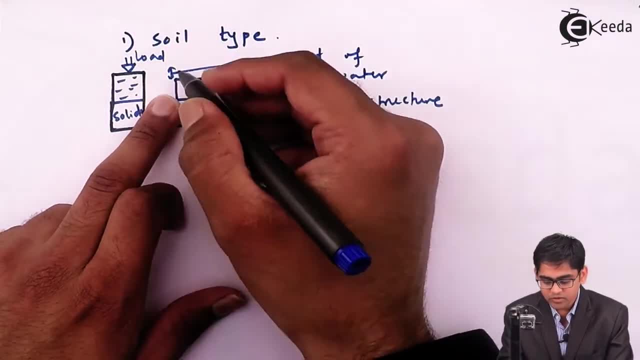 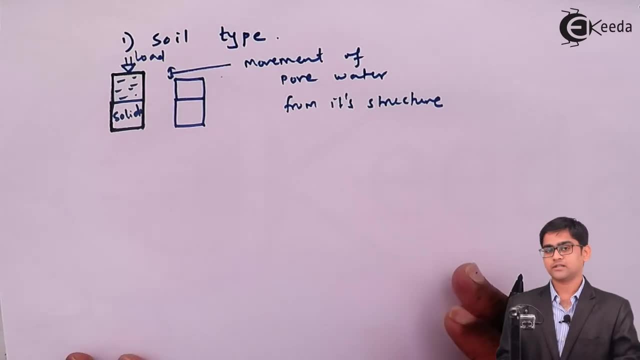 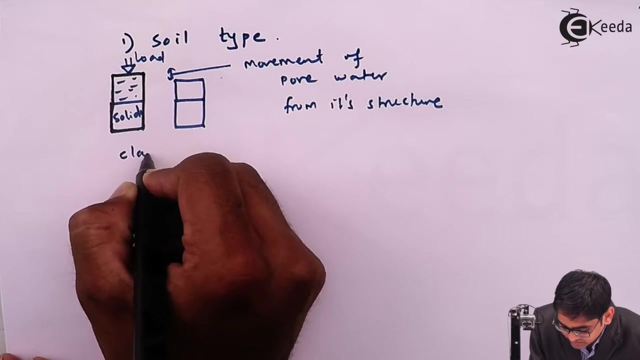 will going to happen. see, the water is moved. that means the flow has occurred. so to occur a flow there has to be a hydraulic gradient, so that hydraulic gradient is generated because of the application of the load. so this particular soil type will depend. so the- particularly in case of the clays- this particular volume change whatever. 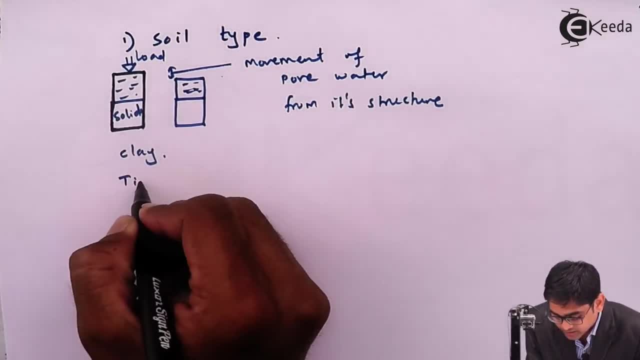 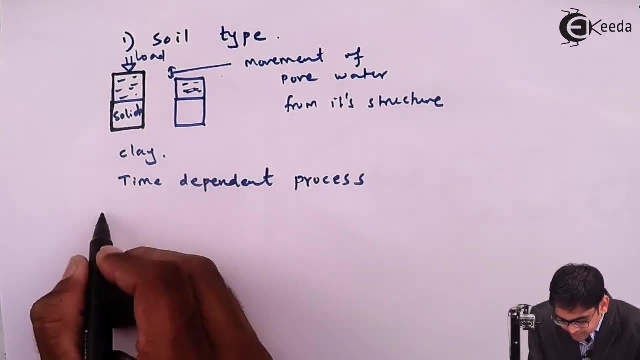 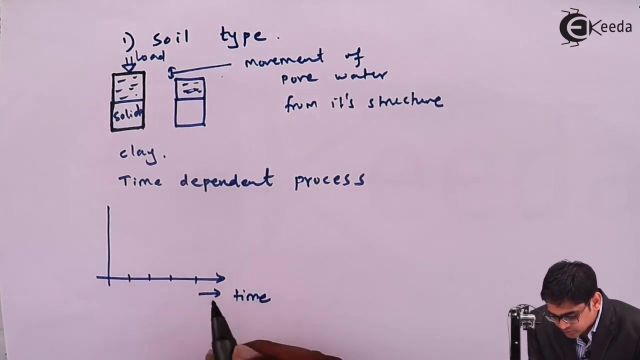 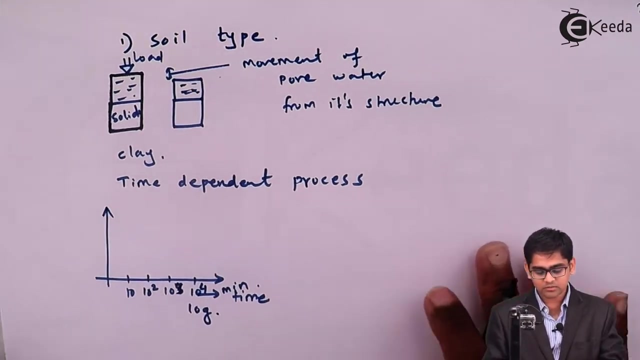 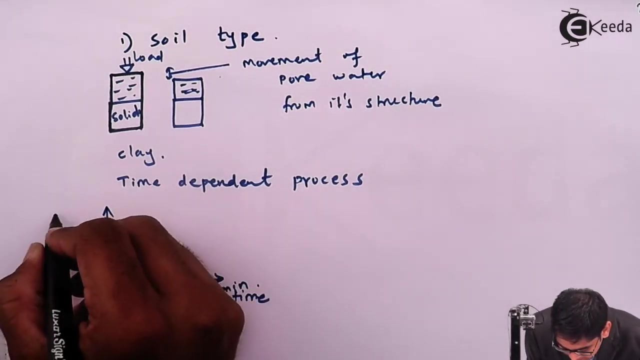 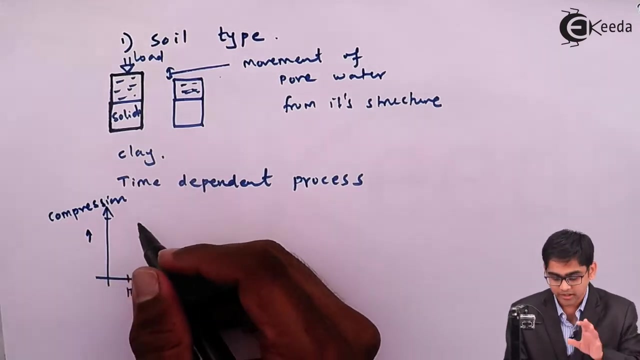 will be happening because of the load is a time dependent process. just, I will deliver it in this table with the number of the blended. so if I just draw a graph of the time on the x-axis i, I will use the log scale over here because, And if I analyze and if I check, it's the small sample of the clay and if I test it in a laboratory and if I just get this on the y-axis as the compression, it is obvious that the compression of the voids only because I am assuming that the solids are incompressible. 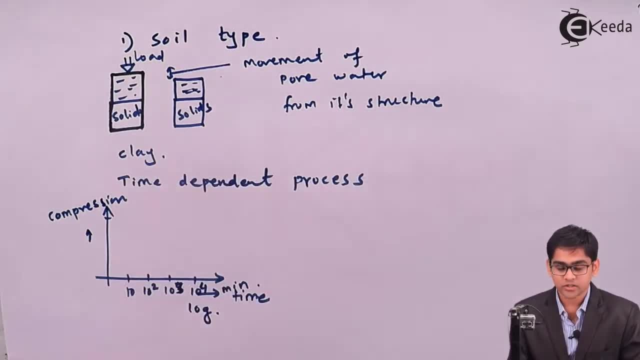 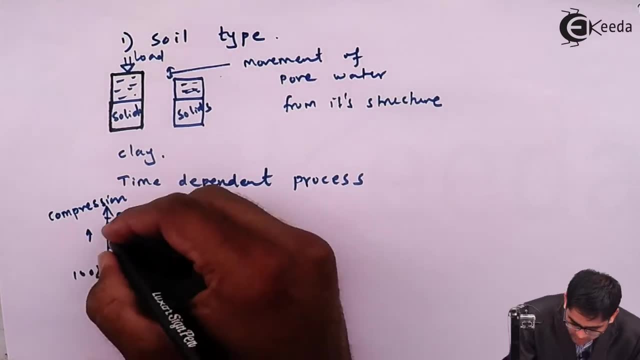 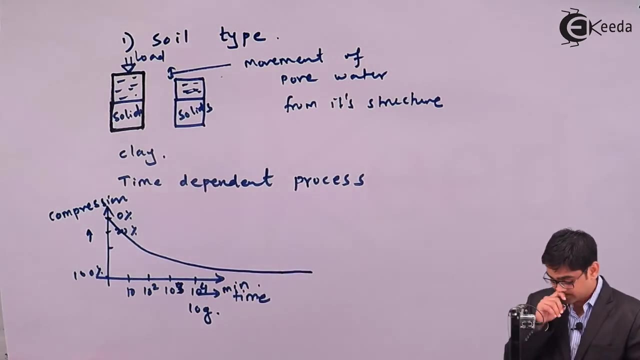 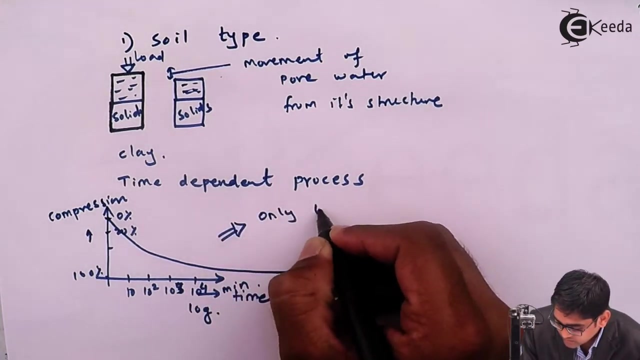 So there won't be any kind of the reduction in the volume of the solids. So over here is a 0%, 20%. So like that, here is 100%. The compression will go on decreasing with respect to time for quite a long period of the time as far as this clay is concerned, because this happens only because of low coefficient of permeability. 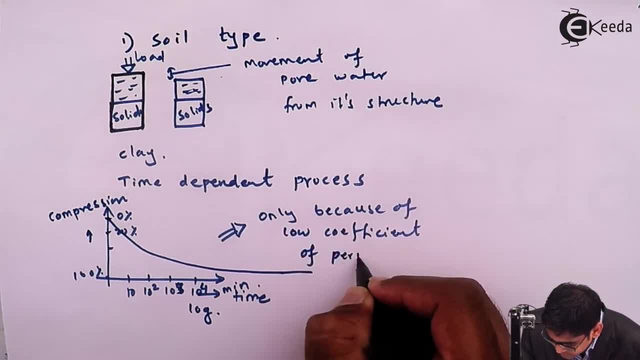 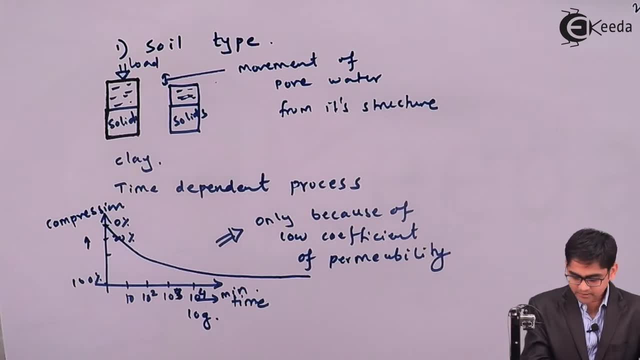 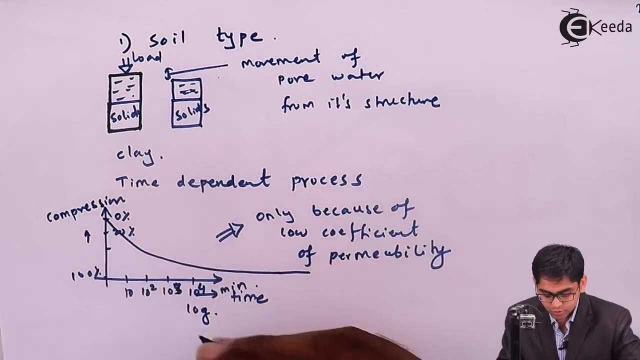 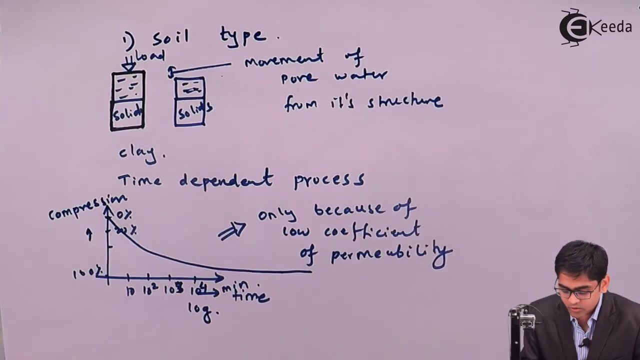 So very, very important. as far as this graph is concerned, we have got the slope of the curve which is gradually decreasing. That means the rate is gradually decreasing. and once you apply the load, what happens? there will be a generation of the load. 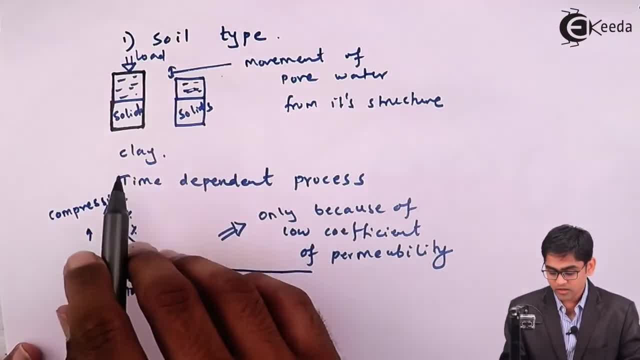 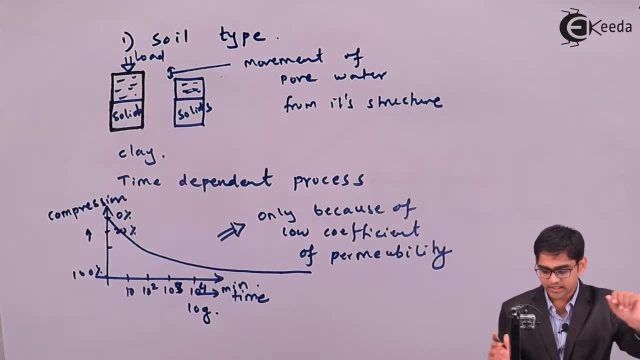 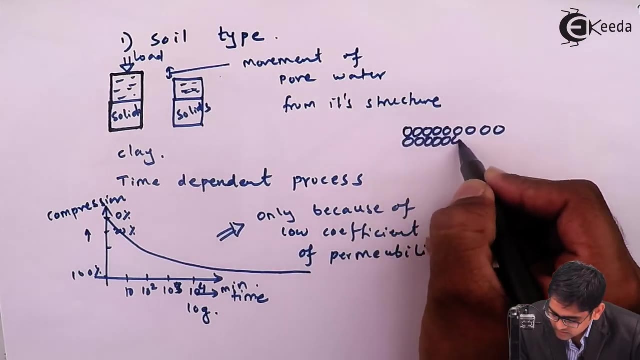 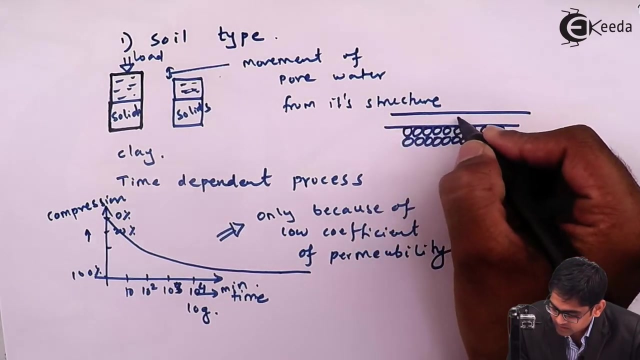 The excess hydrostatic pressure which will lead to a flow condition and that particular flow condition will refer to it as a transient flow condition. So I will repeat again: So if you got the clay particles like this beneath the ground, So let's suppose this is the ground level, This is above, is the. let's consider the clay is sandwiched between the rock and the soil. 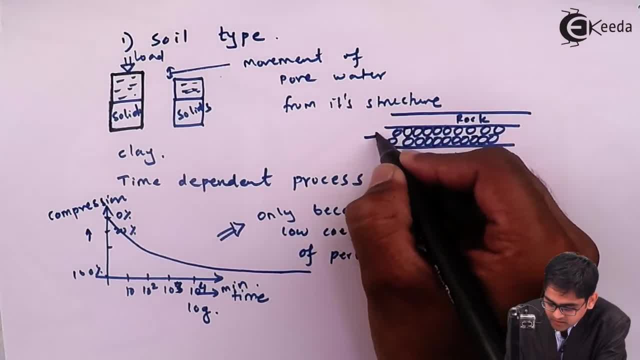 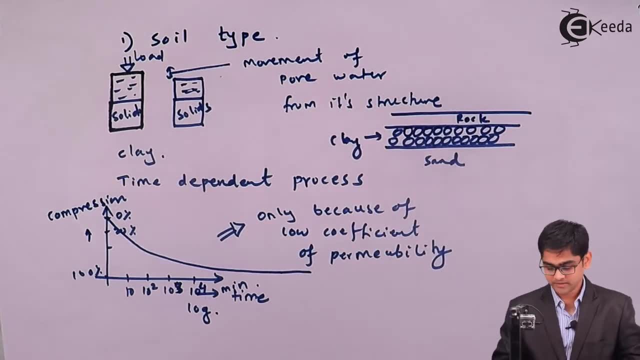 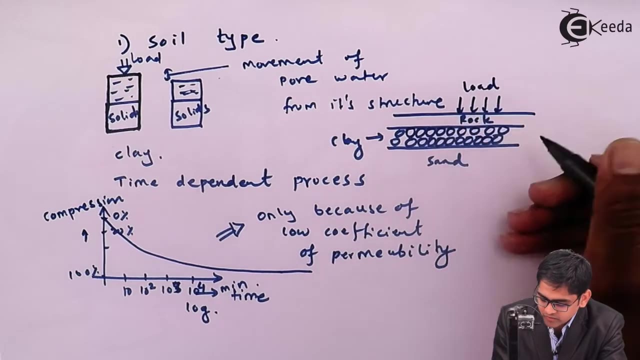 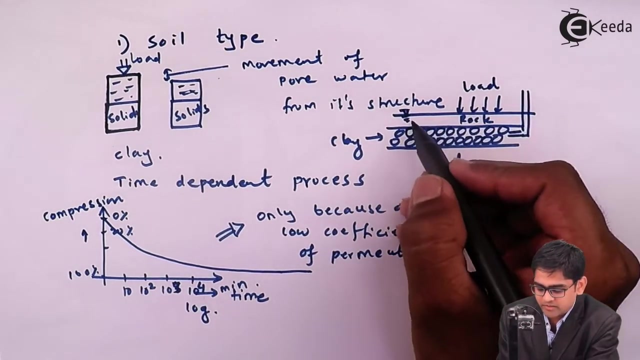 this is the clay. So if I am not applying the load there won't be any kind of movement in the water. So because of the application of the load, this particular load will cause the generation of excess hydrostatic pressure. So initially I consider the water table to be at the ground level. So this is particularly the ground level. 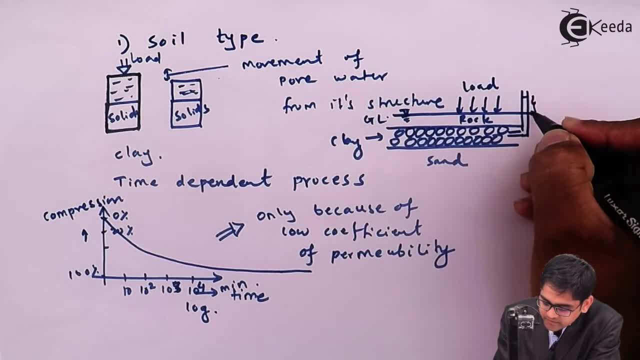 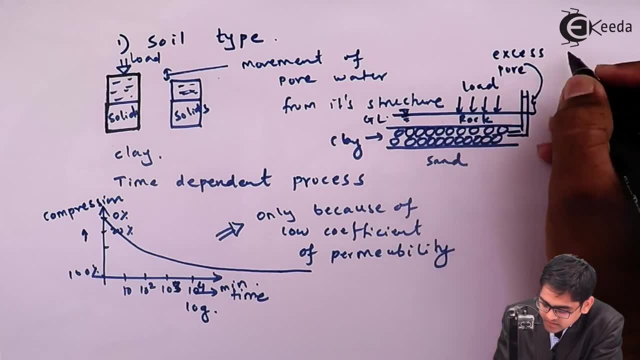 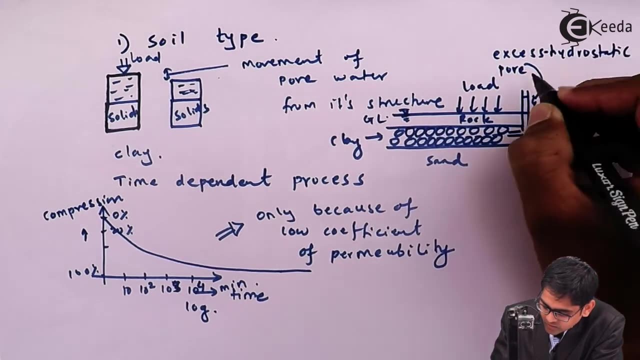 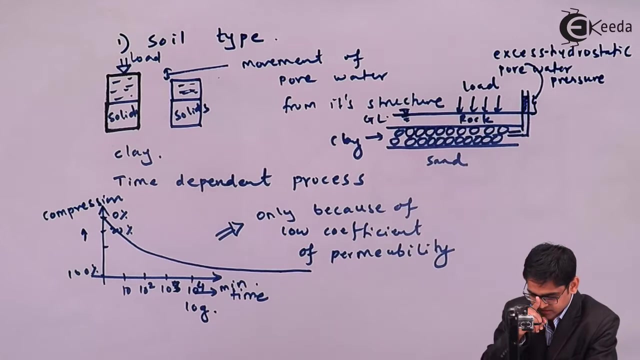 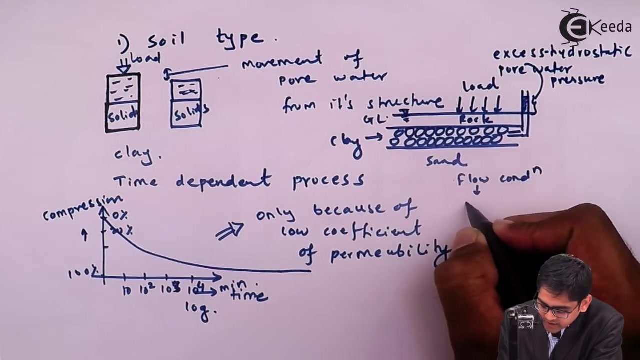 So once you apply a load will be a generation of excess hydrostatic pore water pressure. I will call it as excess hydrostatic, excess hydrostatic pore water pressure. so because of the generation of this much amount of excess hydrostatic pressure, it will lead to a flow condition and that particular flow we call it as a 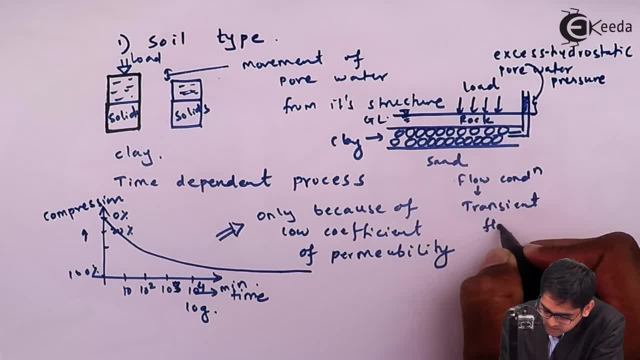 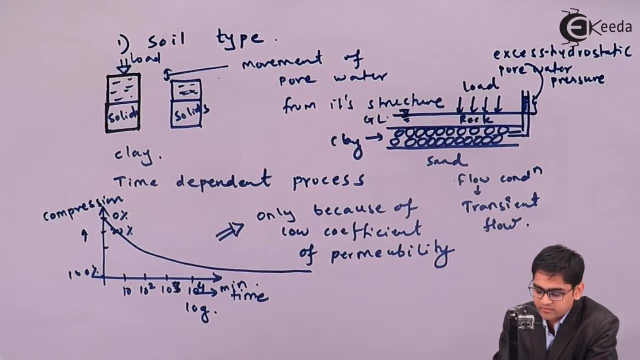 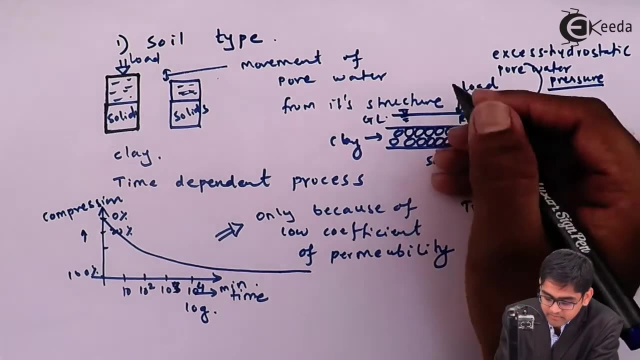 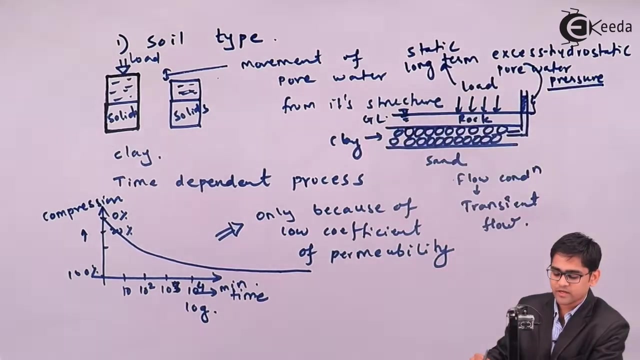 transient flow and transient flow meaning that the flow property will be varying with respect to the pore water pressure which is generated because of the application of the load. so remember this load has to be a static and that to long term, once generated place and you are removed, it doesn't make any sense. so this, particularly the 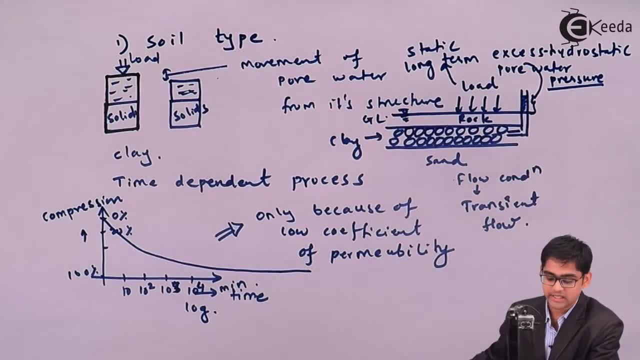 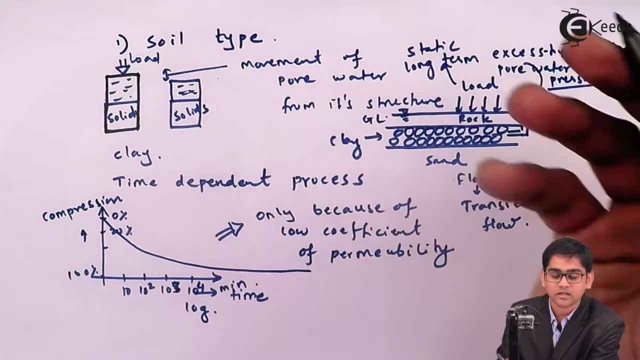 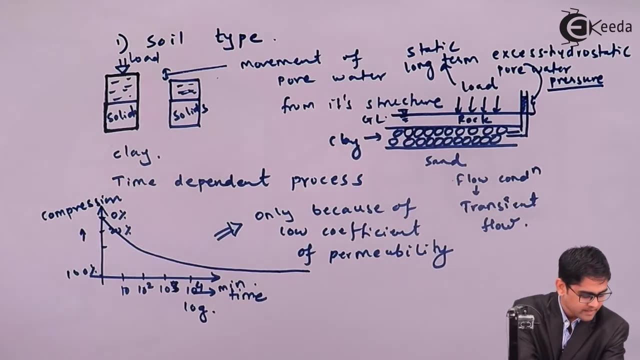 movement of the water or the generation of the pressure, will quickly dissipate. and once the pressure has been dissipated there won't be any kind of the flow condition and there won't be any kind of the moment in the soil mass. so it depends on the type of the soil. so if I just compare the same graph with: 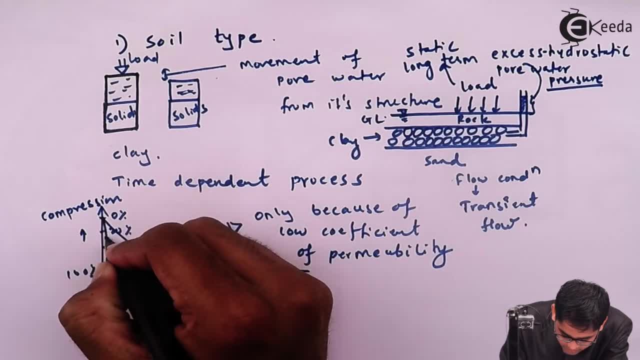 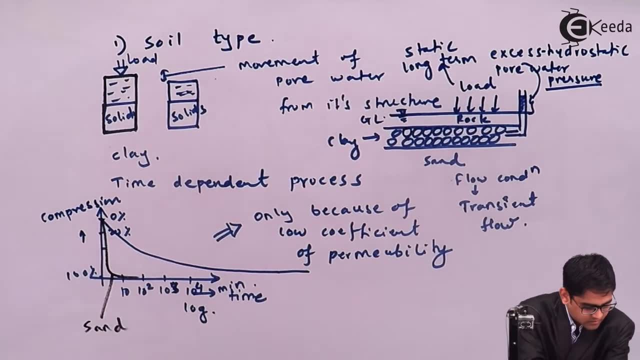 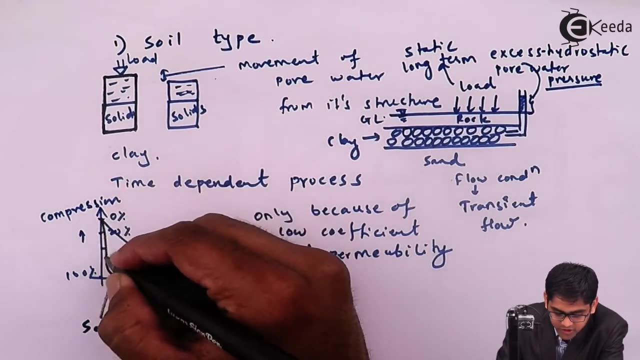 the sandy soil. you will get the response like this: this is for sandy soil. you will get the response like this: this is for sandy soil. you will get the response like this: this is for sand. so in sand, the volume change will quickly occur because of the high 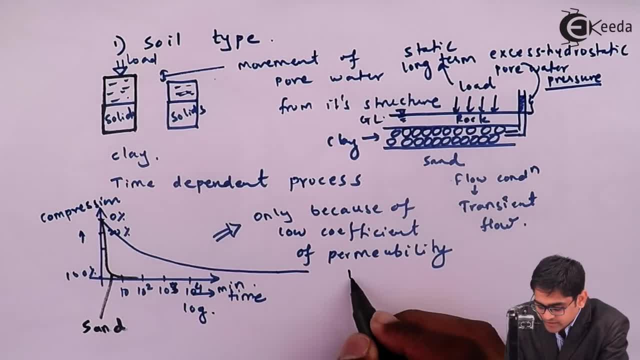 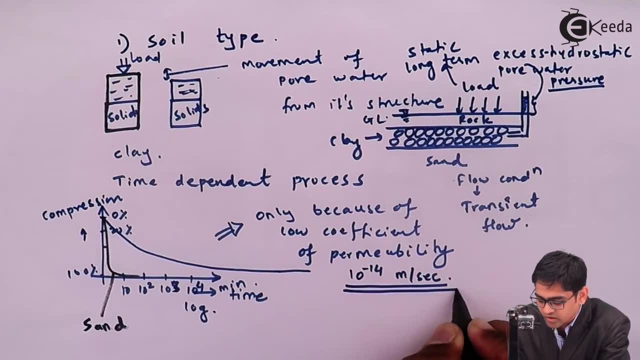 coefficient of the permeability. so if you recollect the coefficient of permeability, that's what we have seen it in the permeability of the soil chapter. for the clays it will be in the order of 10 into 10 raise to minus 4 meter per. 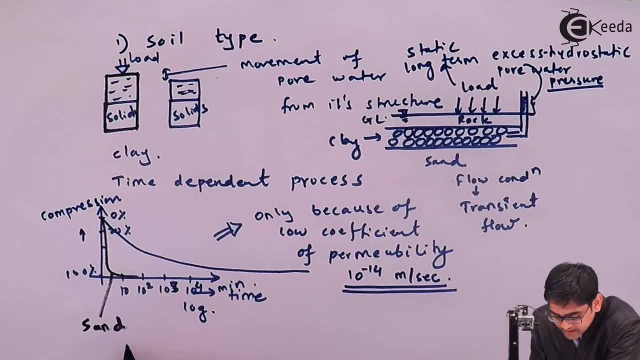 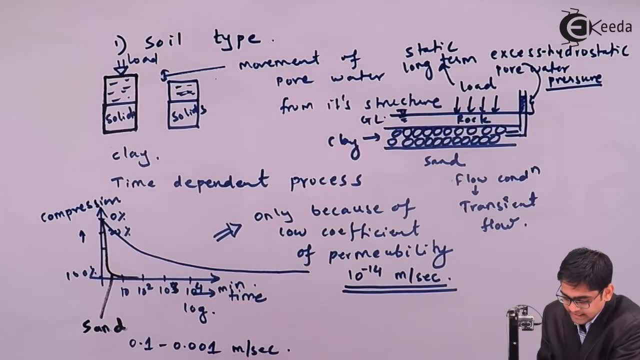 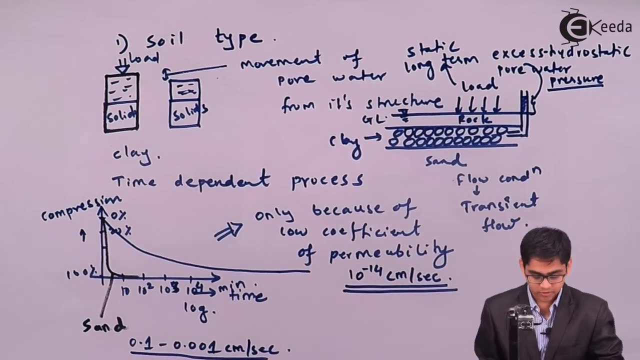 second, while in case of the sands or the coarse grain soil it will be likely to be in the range of point 0,012, point 1 meter per second. sorry, a centimeter per second. that's what we have seen it in the permeability of the soil chapter. so 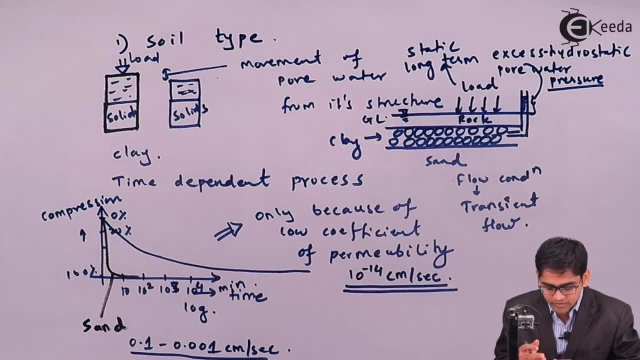 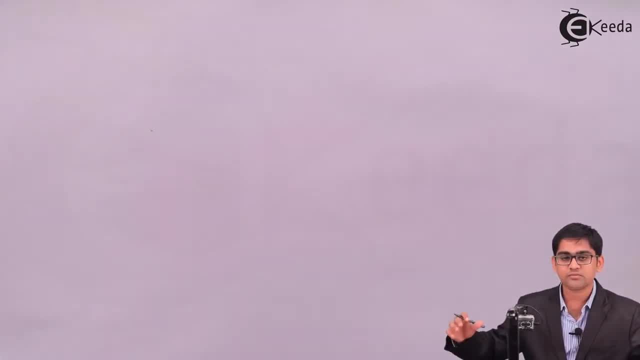 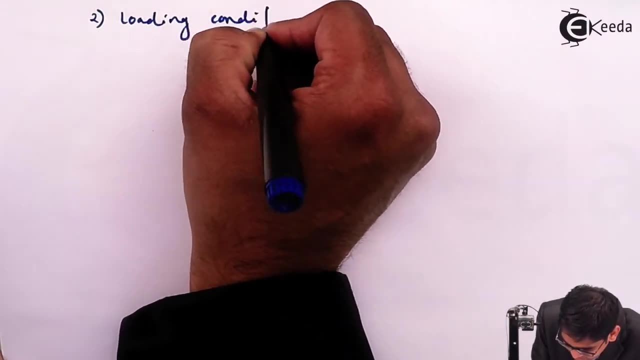 the volume change again will depend on the type of the soil. that's what the first statement, second part, which is influencing the volume change behavior of the soil, is nothing but the loading conditions, and we have seen the how the loading condition will affect the generation of the pore water. 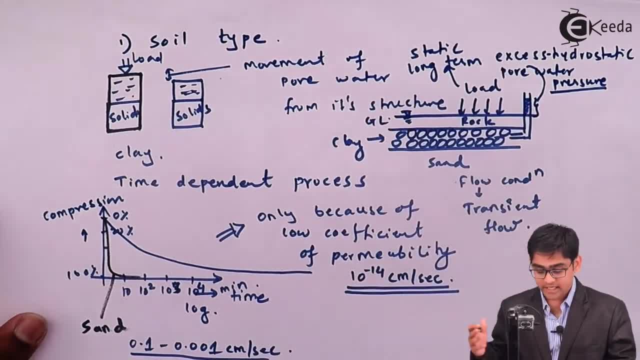 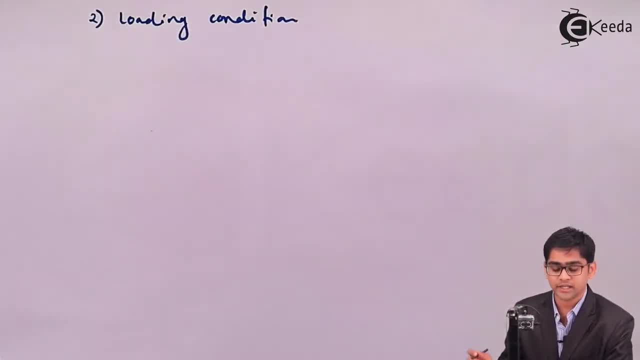 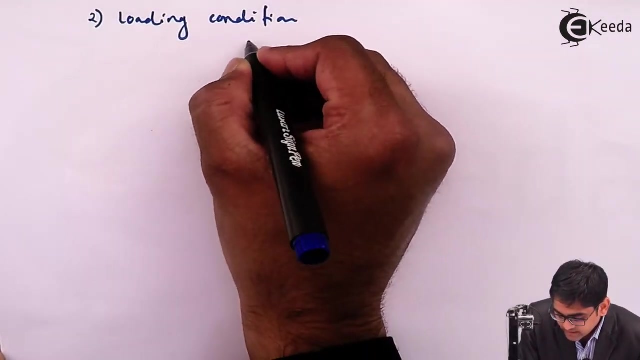 pressure and also the load has to be a static and that to a long term in order to contribute to the generation of the pore water pressure and that will eventually lead to the condition of flow flow condition repeat, so that will eventually lead to a transient flow condition. so we have seen the load to be: 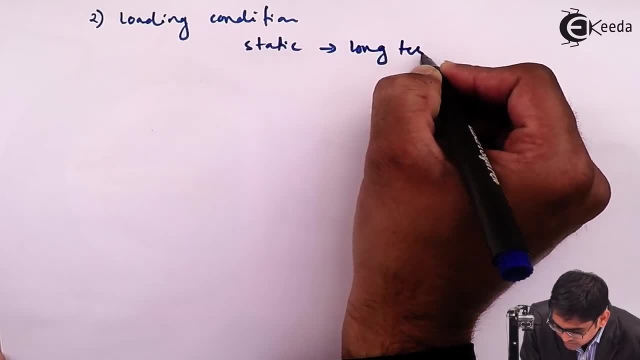 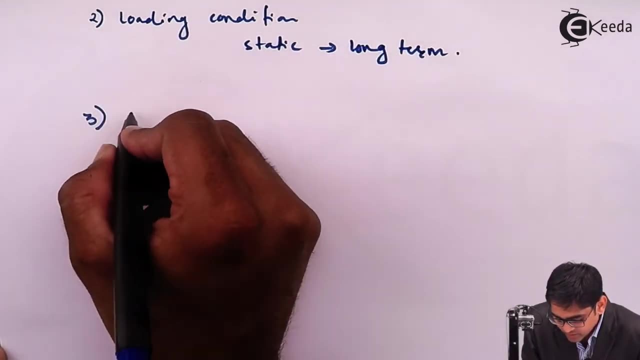 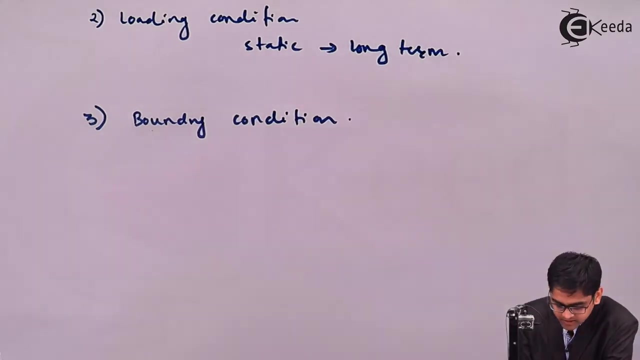 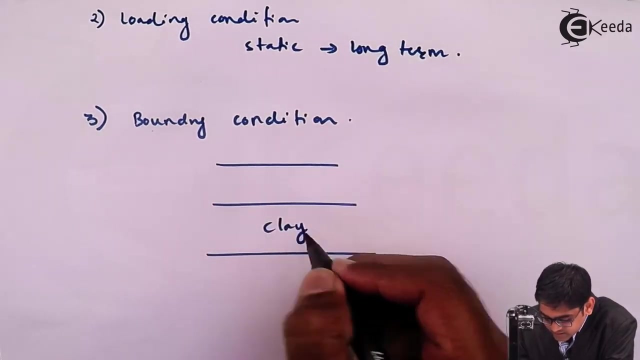 a static and that to a long term, which is contributing this phenomenon called as a change in the volume. and third, very, very important phenomenon will be the nothing but the boundary condition. how the boundary condition will affect, see initially I'll case- I'll consider a clear case- where the clay is sandwiched in between the two pervious layers. 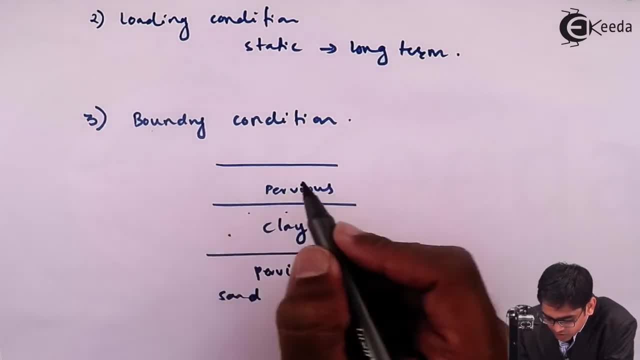 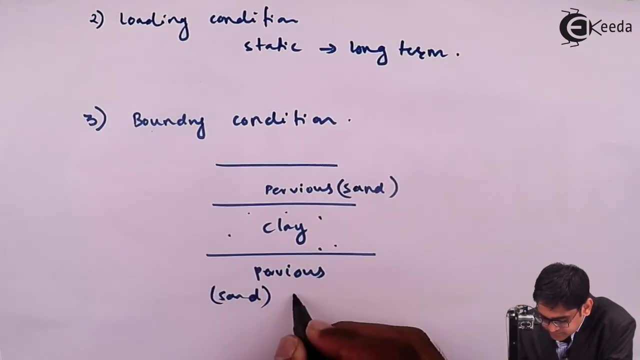 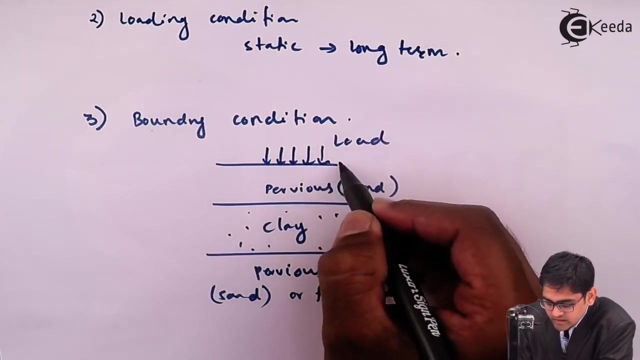 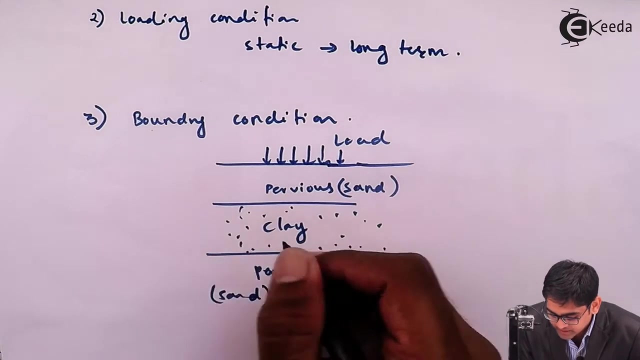 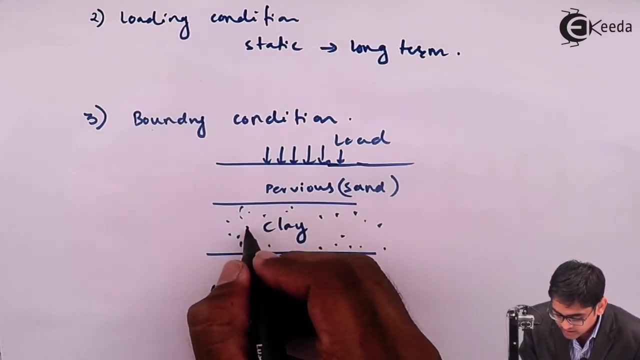 pervious layer may be a sand or the fractured rock, pervious layer of either a sand or fractured rock. and you see, once you apply a load which will generate the excess hydrostatic pore water pressure and, because of the excess hydrostatic pore water pressure, the water in the clay. so remember, whatever clay I am drawing, drawing it in. 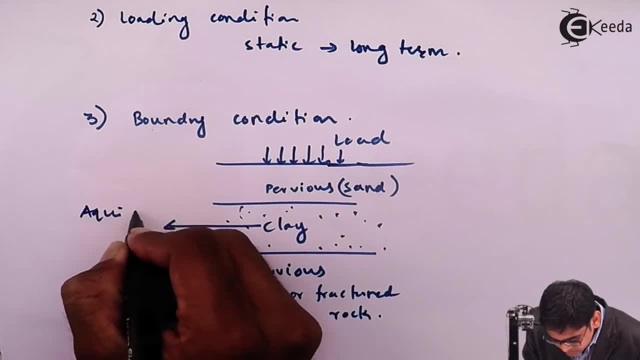 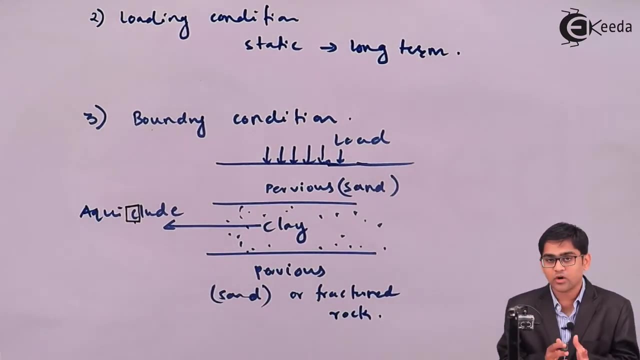 the figure, which means a quick load and because, if you recollect it is in permeability chapter. it is like see, see, clay, clay. you have to match and a quick load. sata contains the water but they cannot yield the water because of the less coefficient of permeability in the 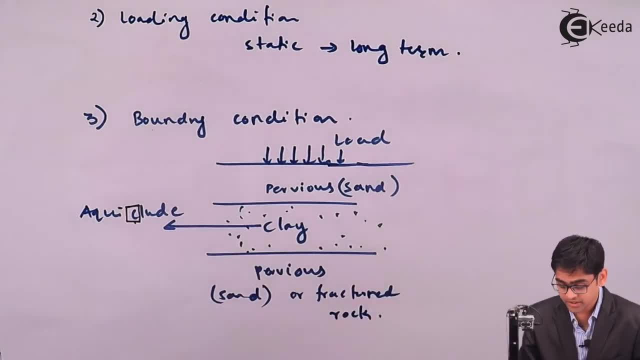 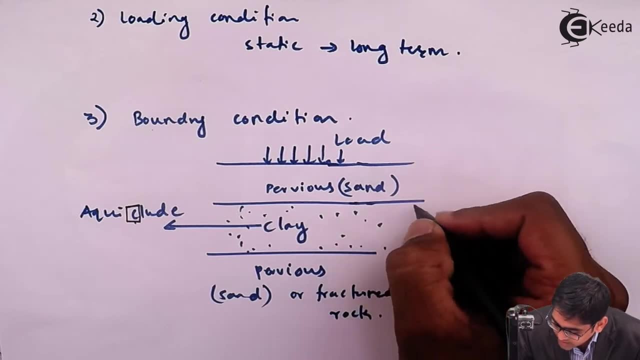 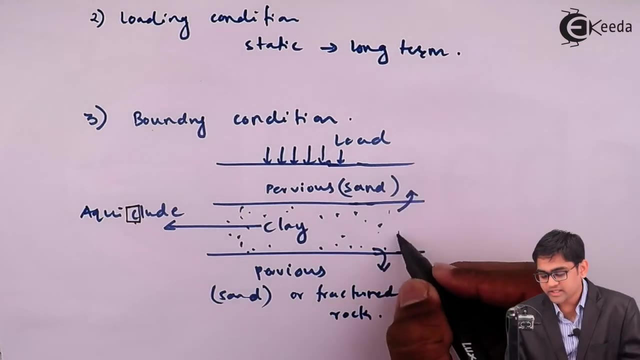 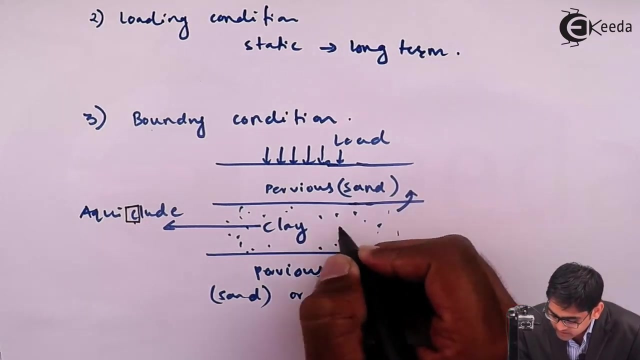 order of 10 raise to minus footing. that's what we have seen in the permeability chapter. so once you apply a load, so the water particle will try to go it into a sand layer and the pressure- that's what- which is generated because of the Lord- will be slowly dissipating. so whatever the thickness of the clay layer, 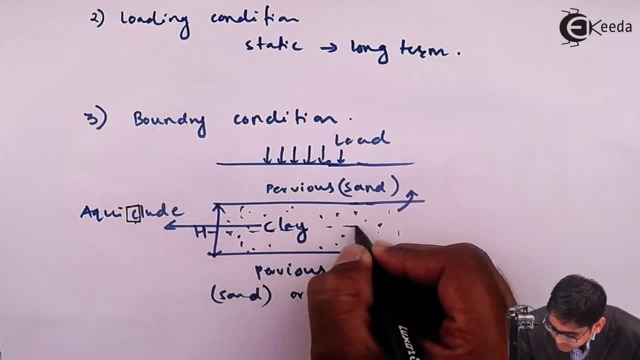 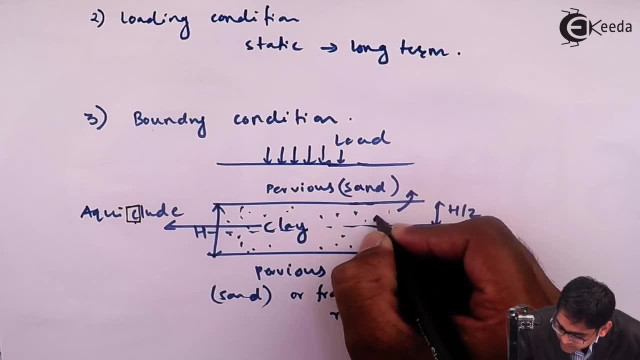 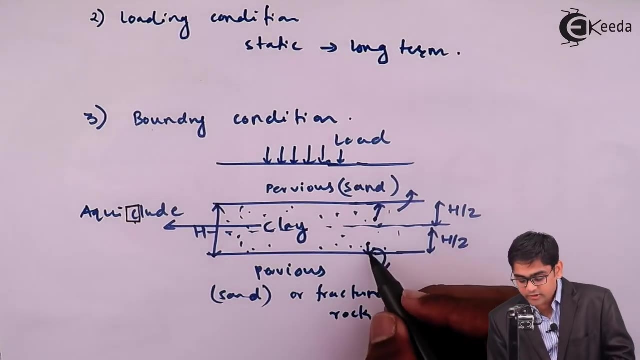 is there, I'll consider the midway of the thickness. so this will be the edge by two and this will be the edge by two. so the water particle which is present here will try to go up side and similarly, the water particle which is there will try to go downside and will try to dissipate all of its energy by going it into a sandy layer. 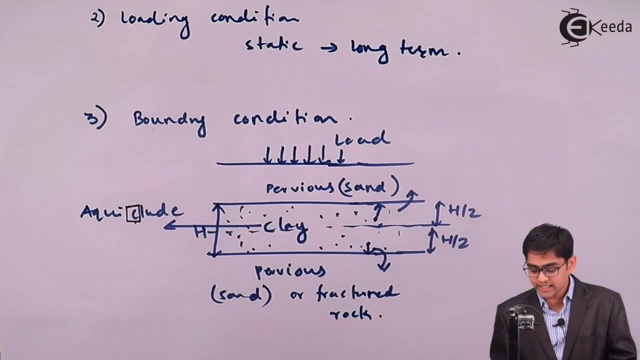 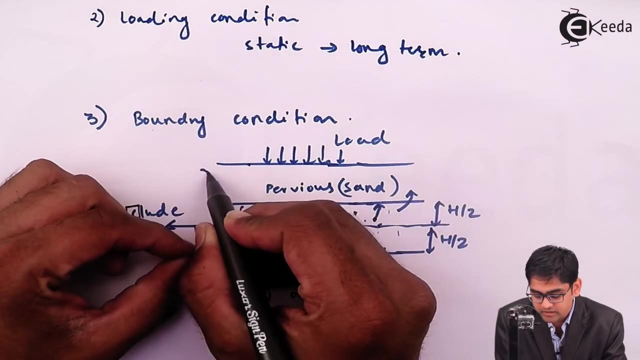 and the sand. since it is a freely drainage available in the sand, it can move along with the force of the gravity. So this is how the volume in the clay will be decreased, which will eventually lead to the surface settlement. So if you plot the surface settlement graph, it would 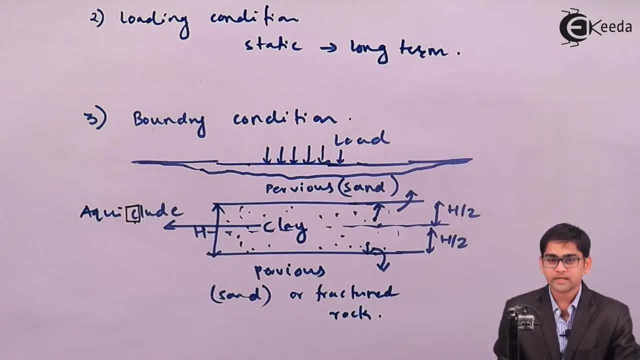 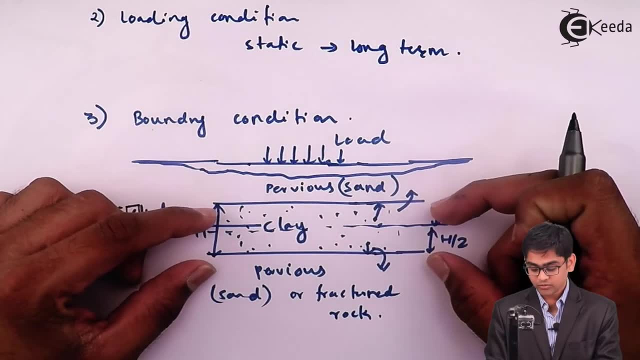 something. look like this: So the area where the load has been applied. you will experience more amount of the settlement if you have got the clay which is deeply buried it into a ground. So this has- this is got the very, very serious limitation as far as geotechnical. 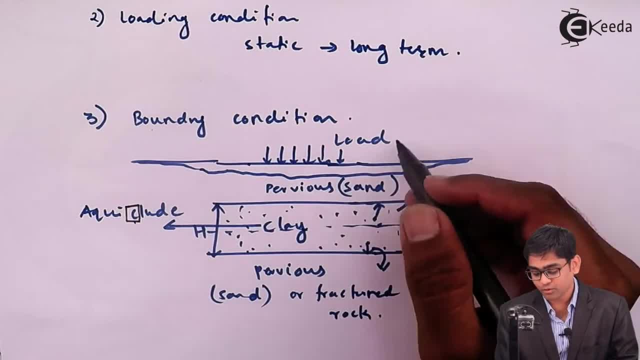 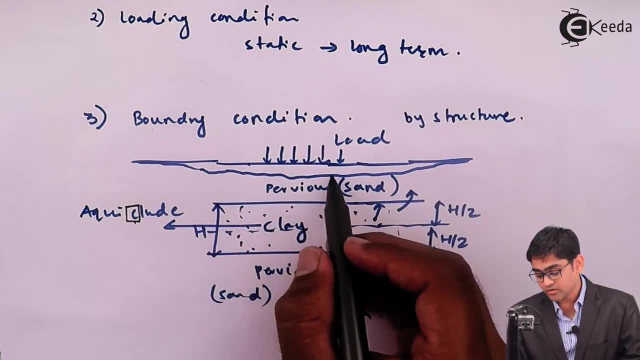 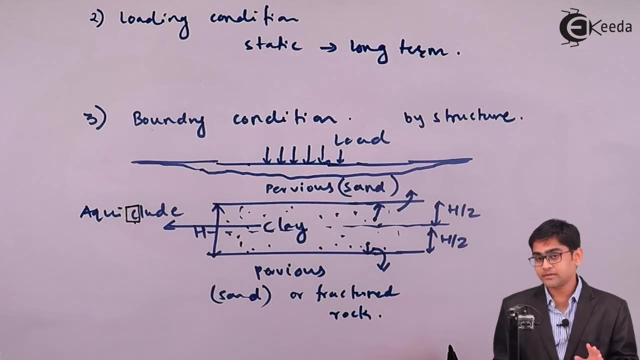 concern because the load is practically imposed by the structures. So you don't allow the structure which undergoes a very, very high amount of the settlement, because it creates a problem to as far as the serviceability, the limited state of serviceability is concerned. 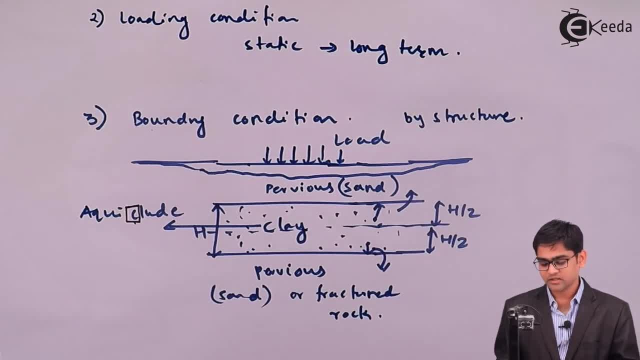 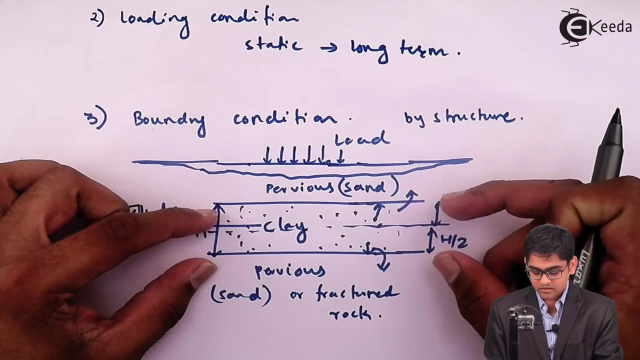 So you cannot allow the very large amount of the settlement to be experienced by the building or the structure. that's what we are planning to have it on the ground. So, as far as possible, what will do it? once you encounter a clay strata, will initially load it.